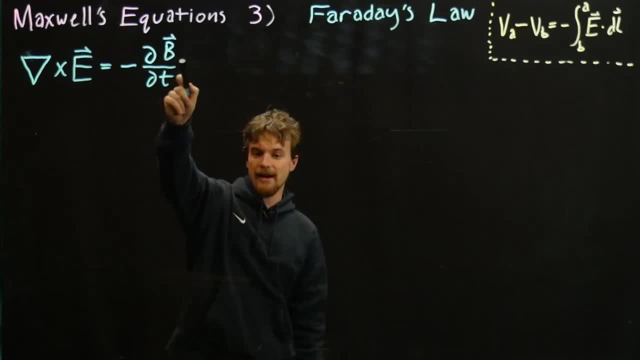 see an electric field term and a magnetic field term in the same equation, and we also see a time derivative in this equation. So now we have some relationship between electric and magnetic field and we'll talk about exactly what it means. but we're into electrodynamics. 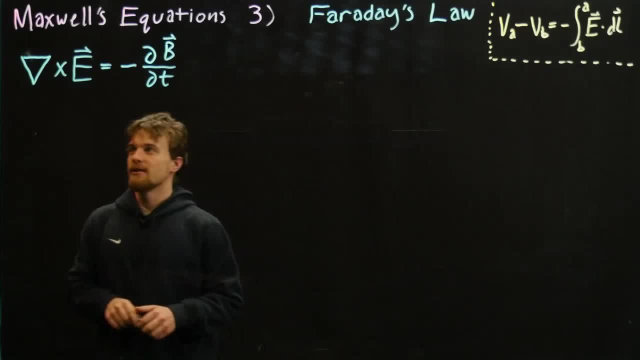 I guess we'd call it So. this equation in calculus terms I guess would say that this operator here is the curl of the electric field. It's kind of the tendency of the electric field to kind of exactly what it says: curl. 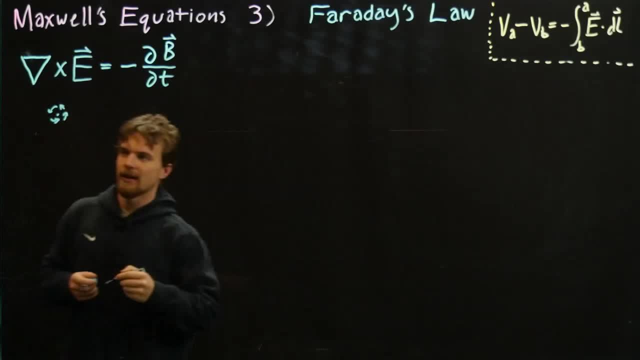 around some point in space and it's a scalar value And this is well the negative of the time derivative of the magnetic field at that point. So this is the differential form and as usual it's a little bit hard to visualize. so we're going to do some integration. 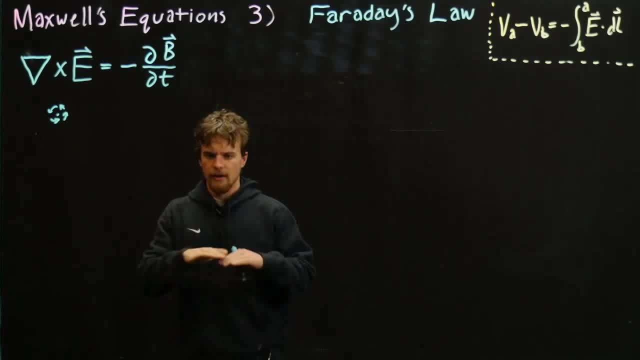 We're going to integrate this into the magnetic field and we're going to integrate it into both sides of this equation over a- let's do it over a surface like a two-dimensional surface or a one-dimensional surface- flat plane. Now, when we integrate this, curl over 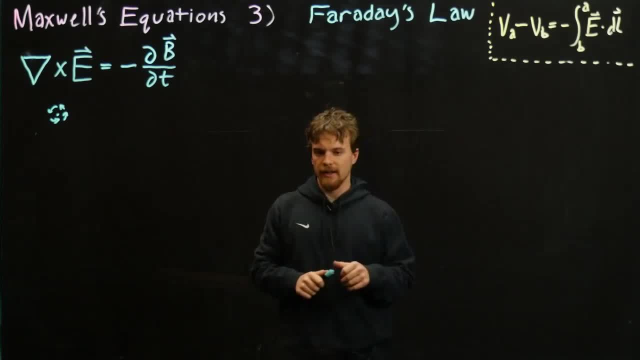 a plane planar surface, it would make sense that the resulting E field in the outside edge would just kind of trace along the outside of our shape, of our plane that we integrate over, And this will become actually- let's just do it So- when we integrate over a two-dimensional. 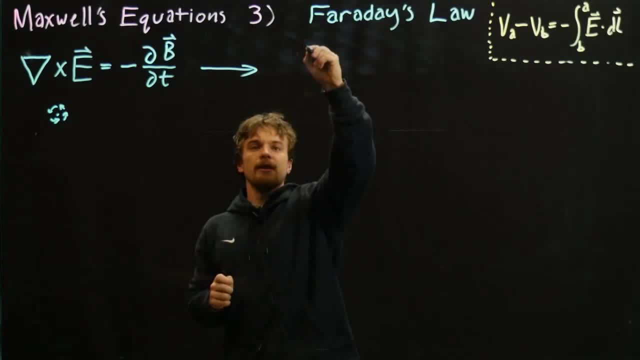 surface we get. this side becomes the integral around the outside, around the outside path of our bit we integrated over And we have there, we have electric field. this side becomes dot product with DL where L is an incremental length along the edge of our shape we integrated. 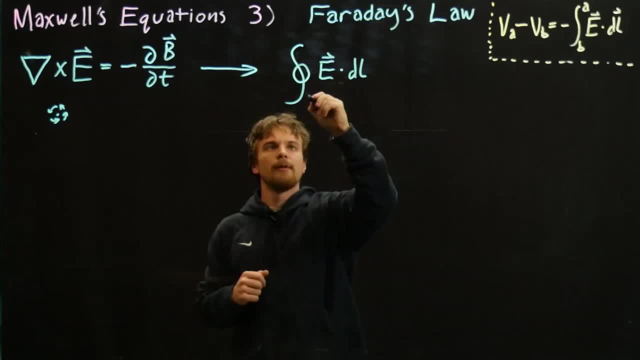 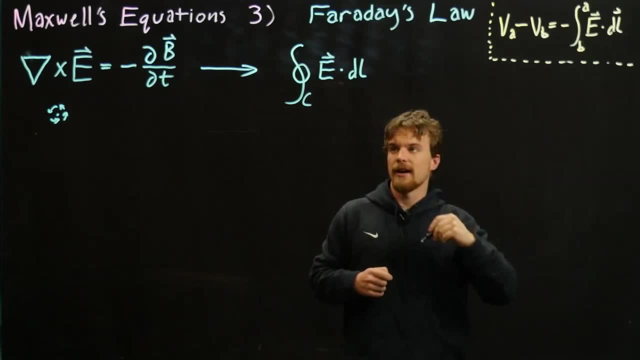 over. So that's this side. that's what that side becomes. Let's call this C. This is just indicating that we're integrating around the outside edge of our shape and that we'll see we can turn that into a circuit. so we'll call it C. So that is all equal to this. 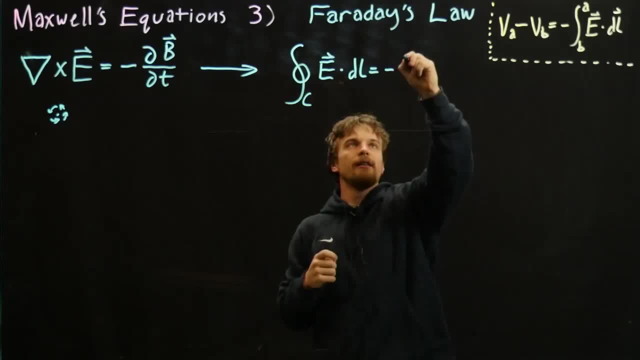 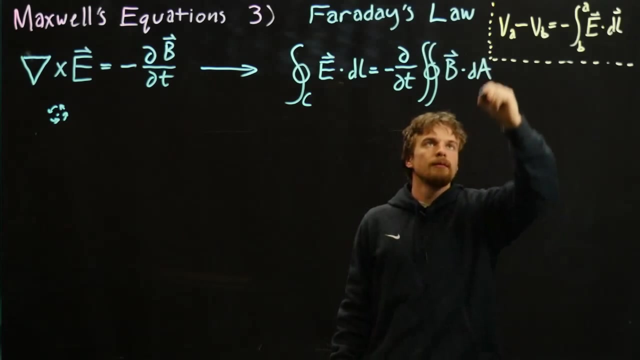 negative sign stays And we can pull this off, Pull the time derivative term out. And now we integrated a B field over a surface, so we get the surface integral of our B field dotted with our differential area. So that is the integral form of Gauss's law. 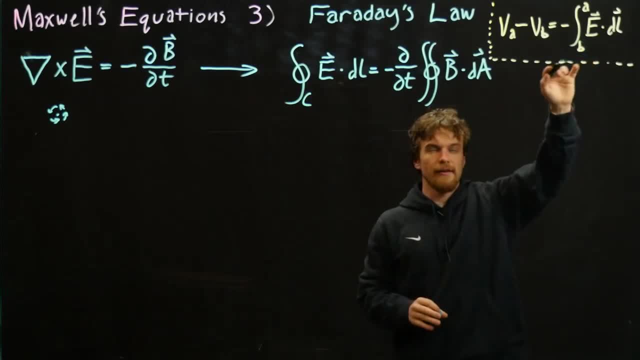 Alright, this is kind of in our way. We'll see that later. This is just the definition of voltage due to electric field. We'll see how that comes into play, But so we'll go like that. So what is this equal to? 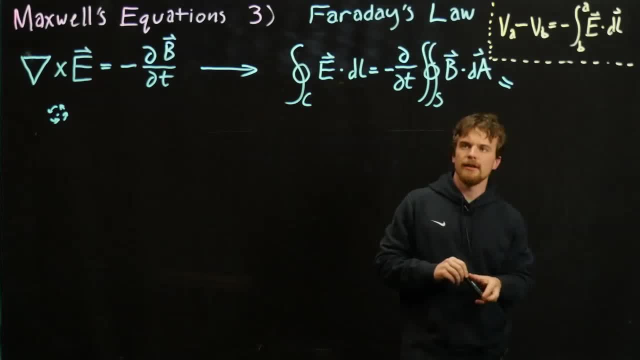 So this is over a surface And we have the time derivative of this term, and this term is the is really the amount of magnetic field That is perpendicular to our surface, Right? So we could call it magnetic flux. So we'll call that, we'll call this whole side of the equation the time derivative of. 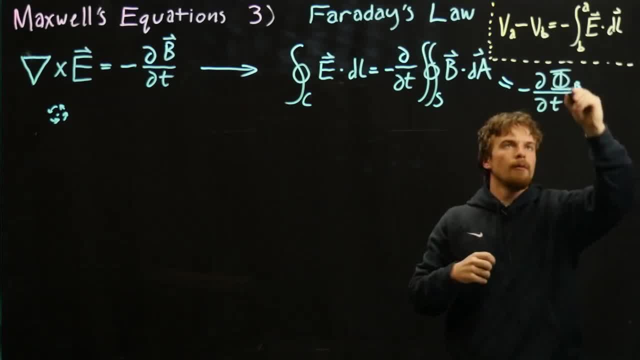 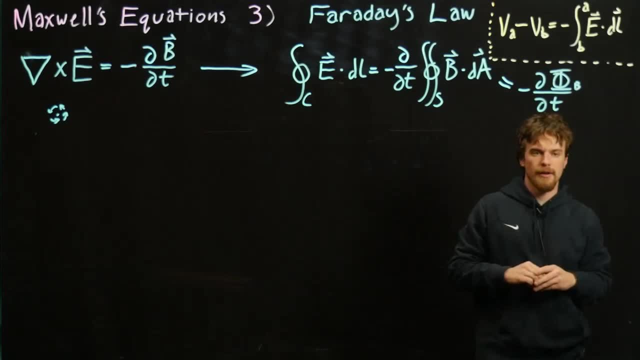 what we call, where this is a term for flux and for a uniform field, say one that is, you know, has at any instant has the same value along our surface. we, integrated over, This would equal to the negative time derivative of B times A, where A is the entire area we. 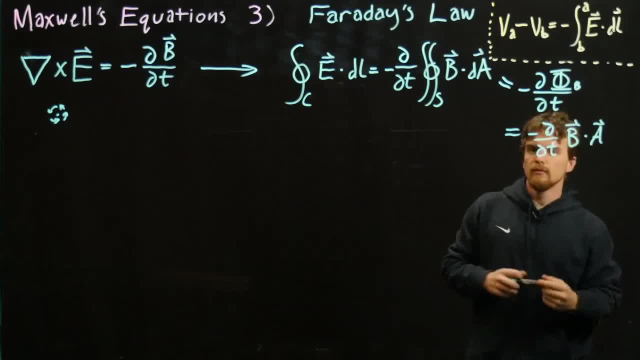 integrated over right. So so this let's do a problem with, with this, Let's do a problem with a uniform, a uniform field. Okay, Let's do a problem with a uniform magnetic field in a in some area. 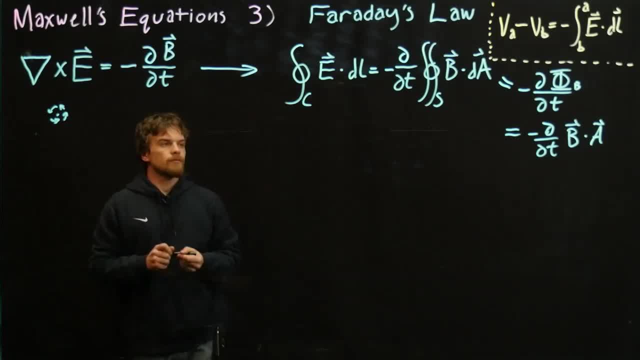 Alright. so let's imagine- actually let's imagine- that we have uniform B field. Now, a uniform B field, one that's at any instant in time, has the same magnitude, that obeys our law. we went over last week Gauss's law for magnetism. 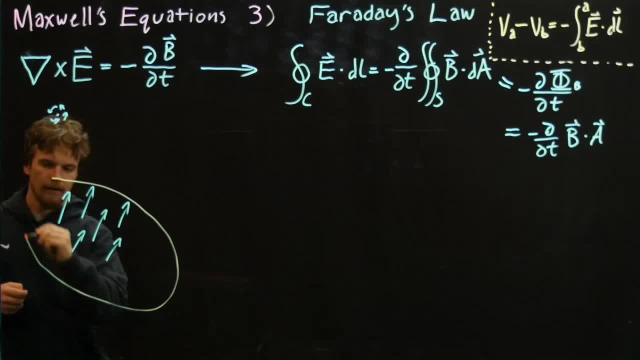 And around this field. let's draw a shape Now. my drawing might not be perfect, but this B field is perfectly perpendicular to the surface of this circle. So let's okay, so let's say that this B field is changing in time, right? 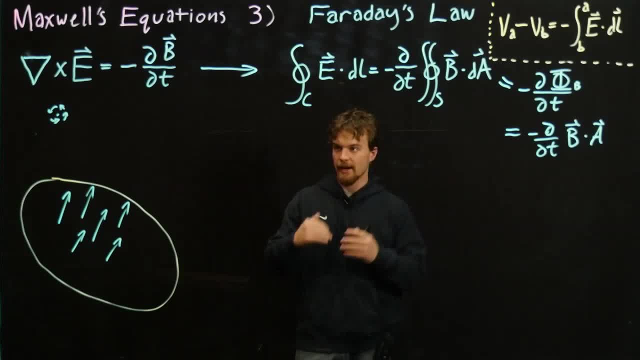 All the vectors have the same magnitude but but they're changing magnitude all together. So we have a time derivative. Let's say this B field is described by. let's say B is equal to five times actually, let's call it sine five times sine of 100 T. Now, that's just something that we're going to do. 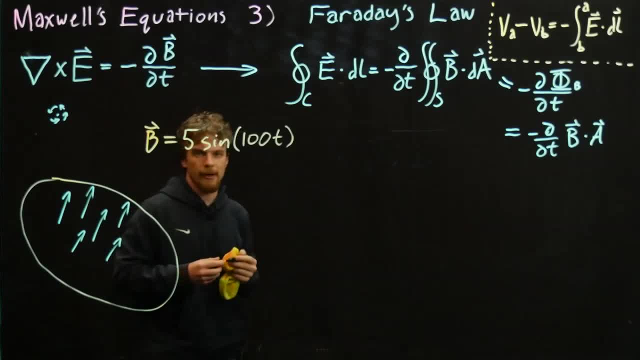 Okay, That's just something we arbitrarily came up with, but that's, that's reasonable. We see sinusoidal fields a lot, And so okay. so the key here is that this, this electric field from a changing magnetic field, it exists all the time. 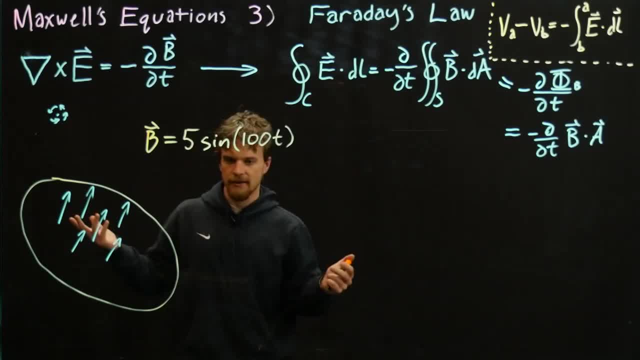 But let's say that this shape we drew, let's say that that's a circuit, let's say that's a conductor. Say we took a wire and bent it around. that way we can make the electric field do things for us. We can move charges around in our, in our wire. 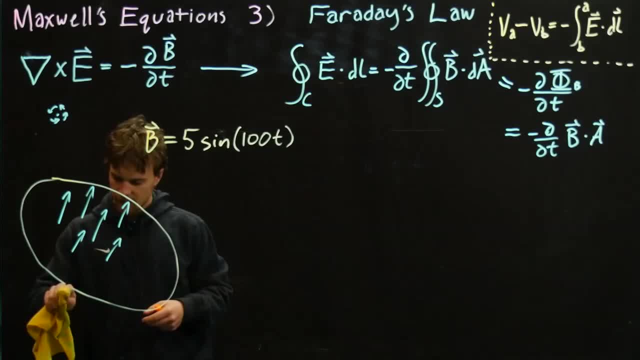 So let's cut the wire just barely, just a little spot right there, And we'll call this point A and we'll call this point B, And now we have an open circuit in between point A and B And we'll try to solve for the voltage between point A and. 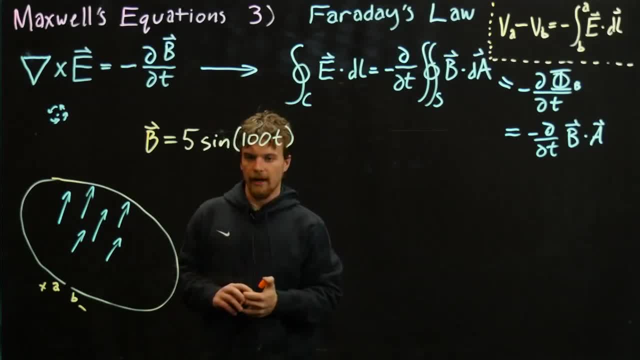 point B: Okay, Okay. So, given that all we know is actually you know what, one other thing we're going to need to know is, let's say, this is a circle and we know it has radius R. So now, given, 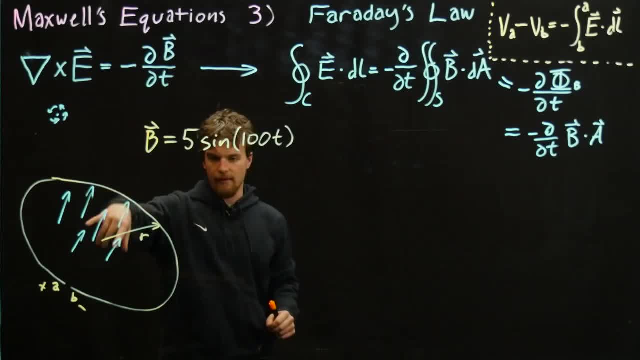 the size of this circle and the value of the magnetic field at any time in it. we'll we'll see if we can solve for this voltage. All right, So so we have a description for the magnetic field, And now, what part of this problem would we like to start with? 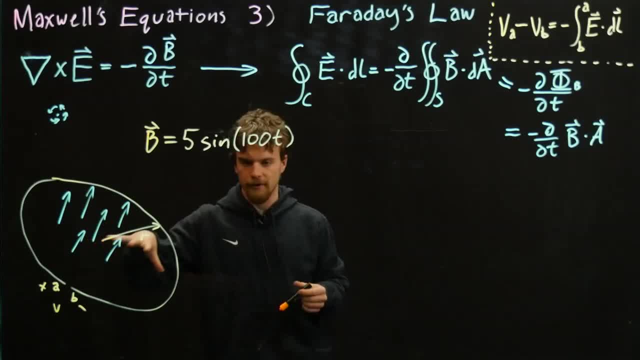 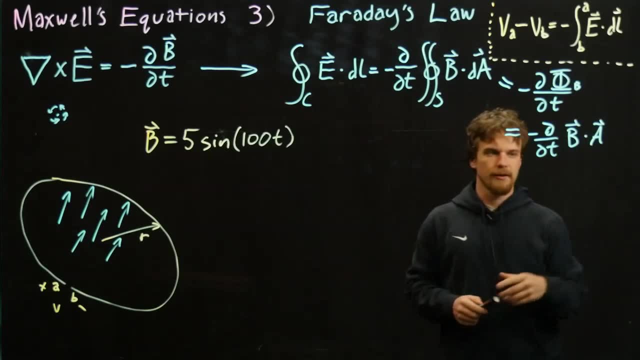 Maybe We know the, the size of our circle, We also know the area of it. So we would know, we could know this term right. We could know the negative derivative of the flux or the magnetic field times area. So we will say that the- let's just come up with a term for just the flux first. 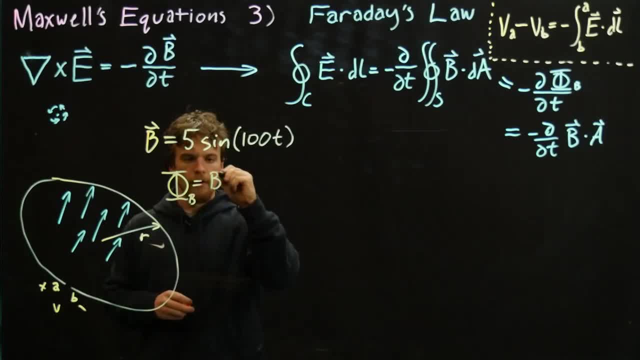 It's going to equal B times A, Where There's a bunch of markers here, Where B is equal to this term. Actually, let's, let's see what A is first. So A- our area, is a circle with radius R, So it's pi, R squared right. 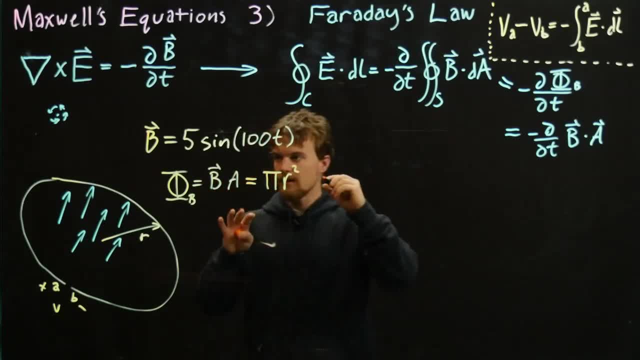 Pi R squared, that's A, And now B is five sine of 100 T. So that's our flux, Okay, Okay. So that's our flux, our magnetic flux through the surface, and we need the negative time derivative of that. 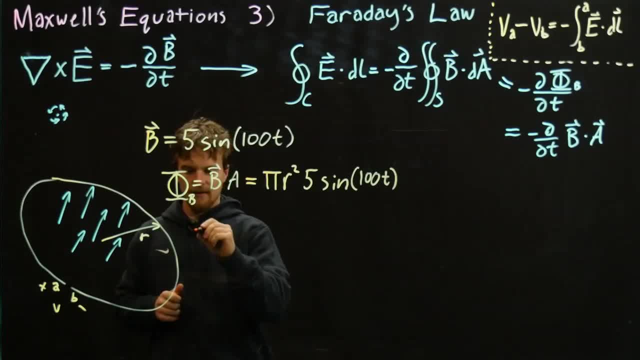 So what is that going to be? That is going to be actually, let's see, it's going to be equal to: so the derivative of sine is cosine, but we want the negative derivative, So we're going to have to say it's equal to negative. 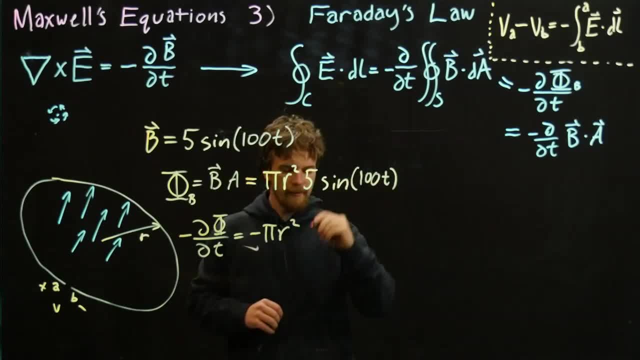 So we're going to have to say it's equal to negative pi R squared 500 cosine of 100 T. Does that make sense? So we just, yeah, we took the negative time derivative of this term right here. So what is that? 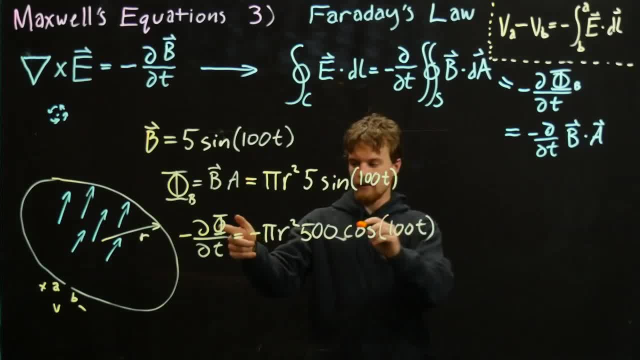 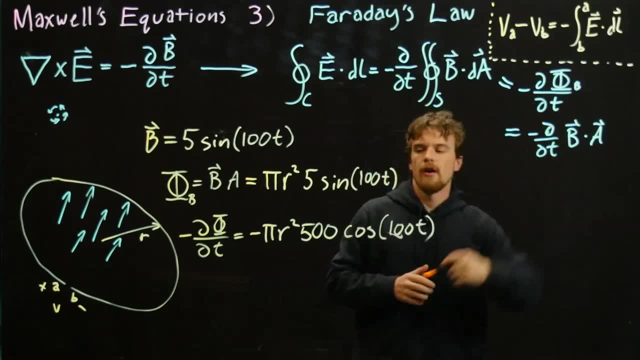 This, according to Faraday's law, this entire term. right here is this term, So now we could set it equal to the other side of this equation. Let's see. Okay, actually, one other thing that's pretty important. We have a convention called the right hand rule. 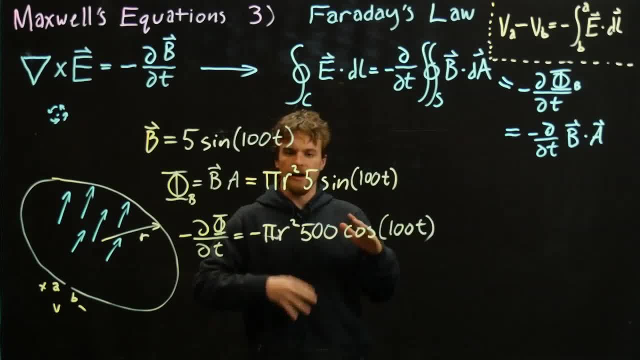 Now what that says is that this: it's kind of arbitrary how we define this direction, this differential direction and this differential area, but the right hand rule says that if we define the differential area to be this way, which we did, then we take the thumb. 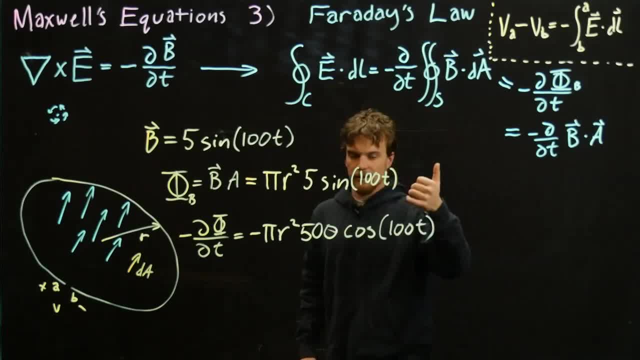 of our right hand. We point it in the direction of our differential area, and the way our fingers curl is the way we integrate the line, the way we do this line integration around this. Does that make sense? So now we have a term for the negative derivative of the flux and we'll do that integration. 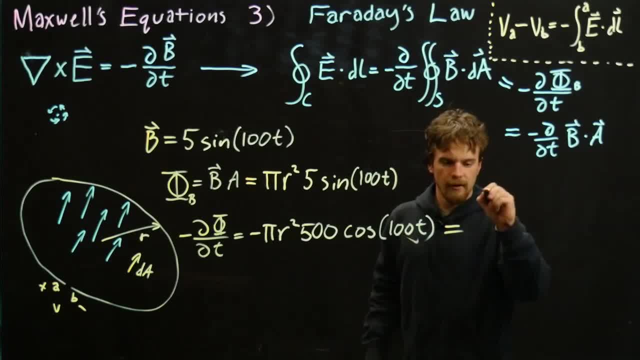 We can say this is equal to the integral. and which way do we go? According to the right hand, According to the right hand rule we want to go. we want to start at B and go to A, right, So this would be the integral from B to A of let's see our electric field that exists. 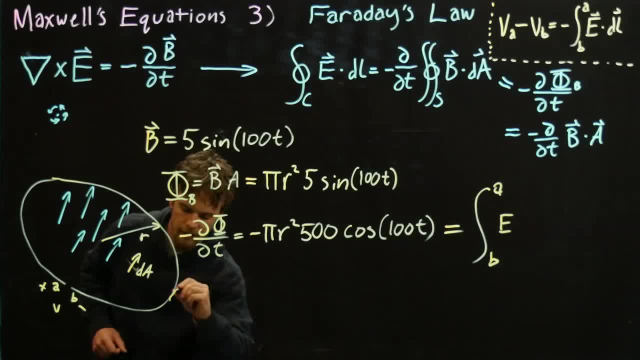 along this outside and our, so our DL would be pointing in this direction: E dot DL, So that way. Okay, So that looks pretty familiar from our definition of what voltage is right. So we look up here and we see that in any two points in space VA, the difference of 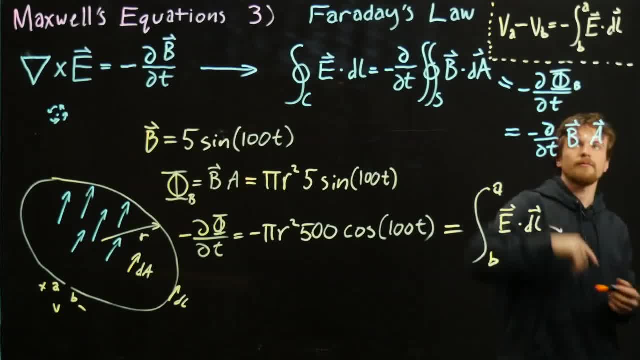 the voltage at any two points of space, VA and VB, is the negative integral from B to A of E dot DL. That holds for any path we can make through any electric field. So we kind of we have that almost here Yeah. 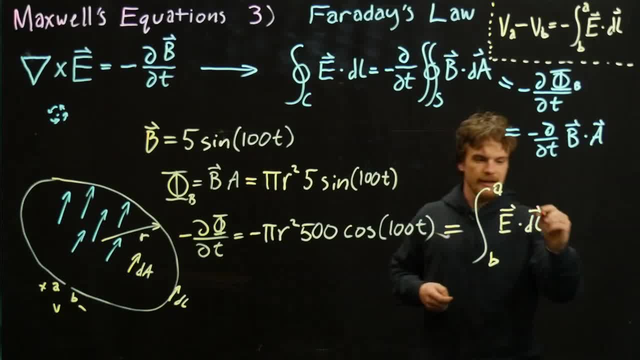 It's just missing a negative sign, right? So if this is equal to the negative voltage between A and B, right, then we can say that the voltage between A and B is equal to the negative of this term by R squared 500 cosine. 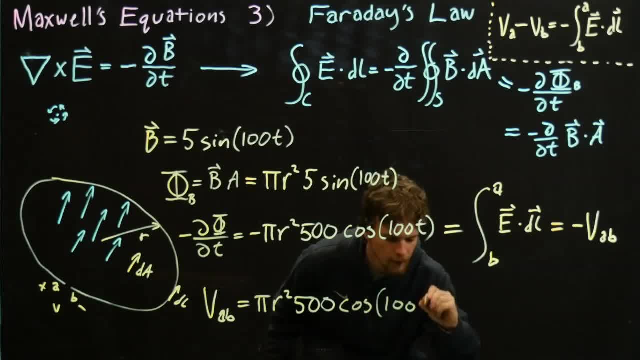 of 100.. Okay So, and this is the same thing for A and B, so we can get the value of this 500 T Alright. So basically, we're saying that, given this electric, given this magnetic field changing through this surface, we would see a voltage at this value in between points A and B, And